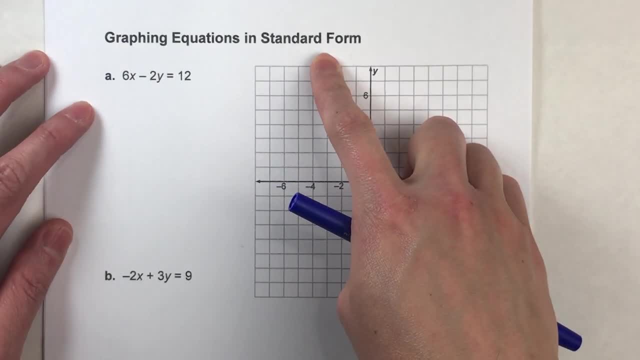 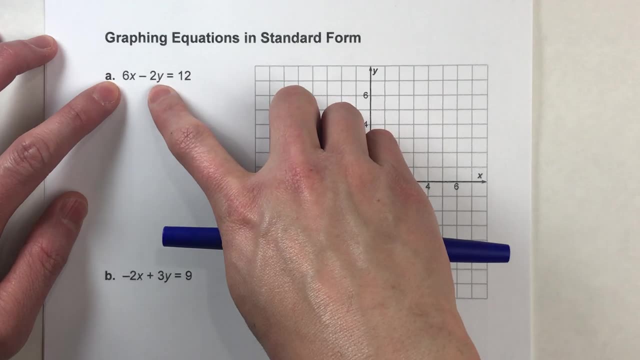 So today we're going to be graphing equations in standard form. Now, these two equations are examples of equations that are in standard form. Notice, we have x and y on the same side of the equal sign, equal to just a regular number on the other side. Now, we're not used to graphing. 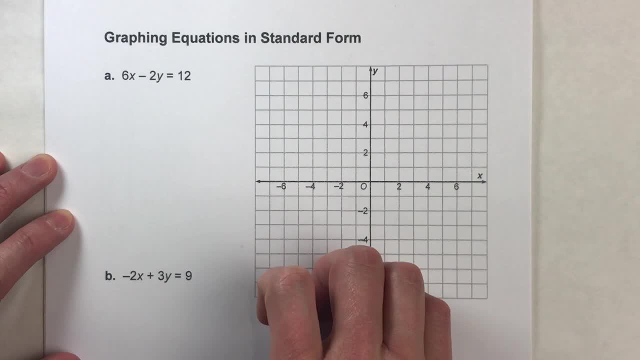 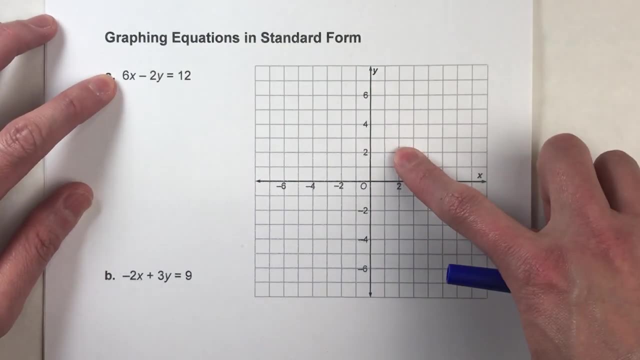 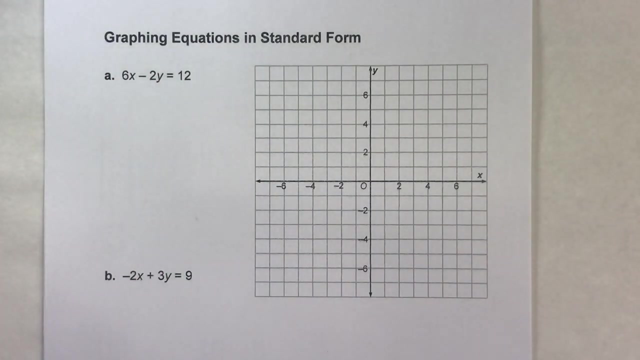 equations in standard form. We're used to graphing equations that are in slope-intercept form, that tell you the slope and they tell you the y-intercept. These ones don't do that, So we can't just graph this from just looking at it. However, we can use algebra to get this into slope-intercept. 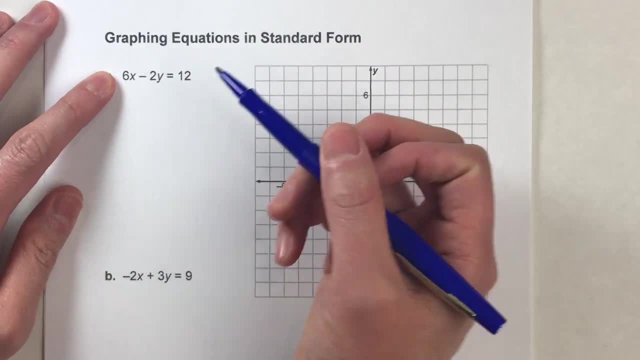 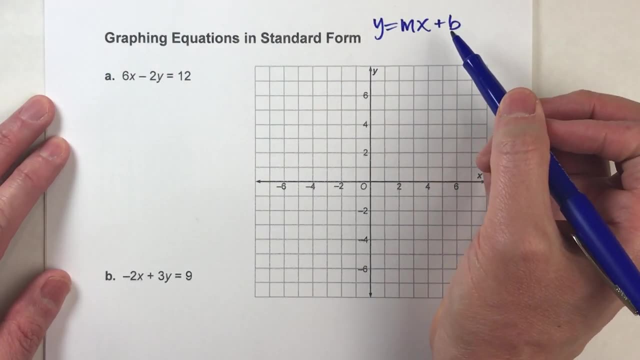 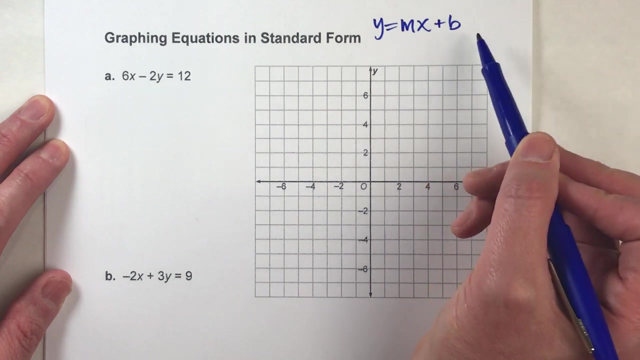 form, and that's what we're going to do. So remember, slope-intercept form looks like this: y equals something x plus something, y equals mx plus b. So if we can use algebra to rearrange this to look like that, then we'll know what the slope is and we'll know what the y-intercept is, and then 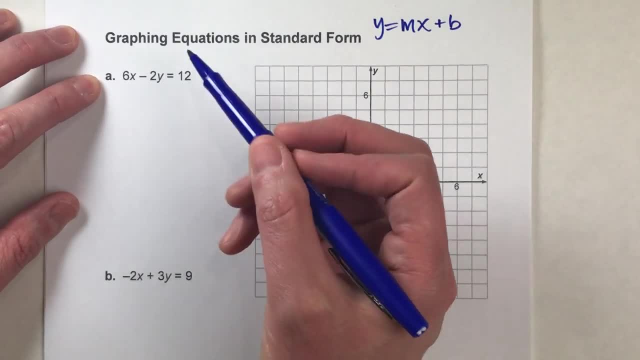 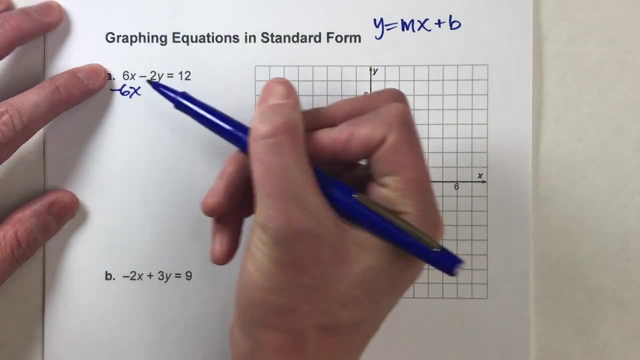 we can graph it All right, So let's do that to this one. 6x minus 2y equals 12.. I want to get the y by itself, So I'm going to start by subtracting 6x from this side. What I do to one side, I have to do to the other, So let's. 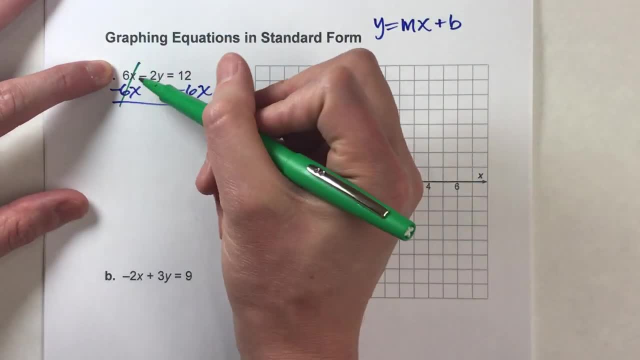 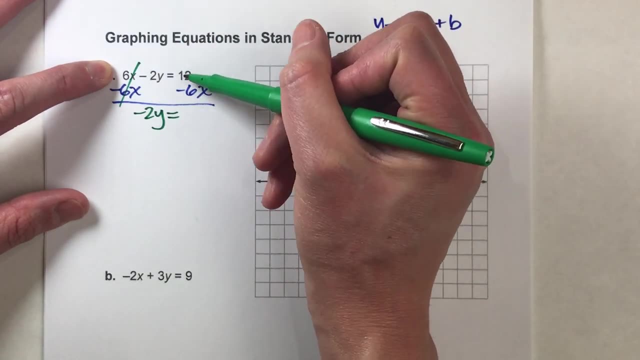 do that, All right. The 6x's on this side don't do each other, but the negative 2y drops down, the equals drops down and notice I can't subtract 6x from 12.. So I'm going to keep these two things. 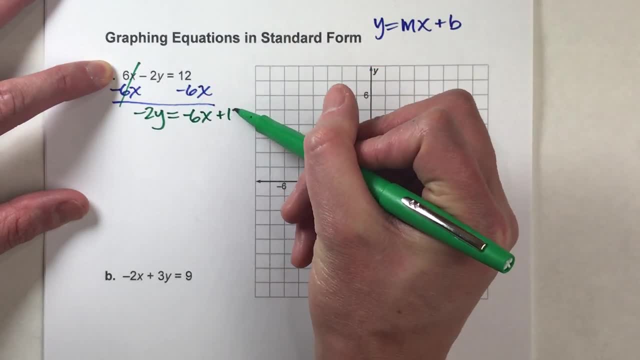 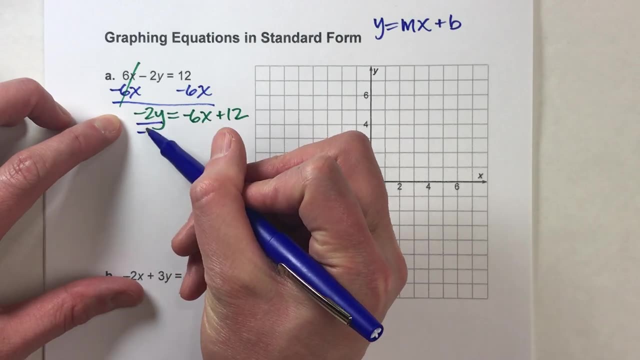 separate. I'm going to keep the negative 6 here and then the positive 12 right here. All right, I've almost got y by itself, but it says y times negative 2, so I'm going to divide by negative 2.. 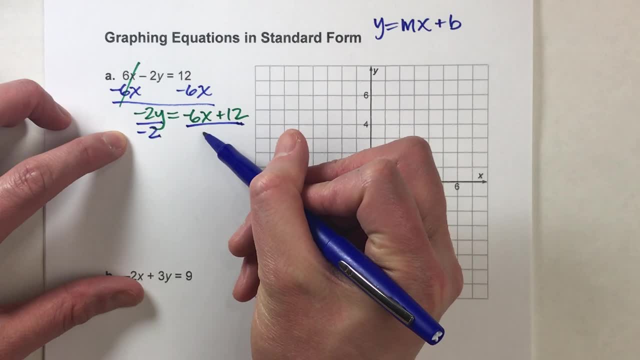 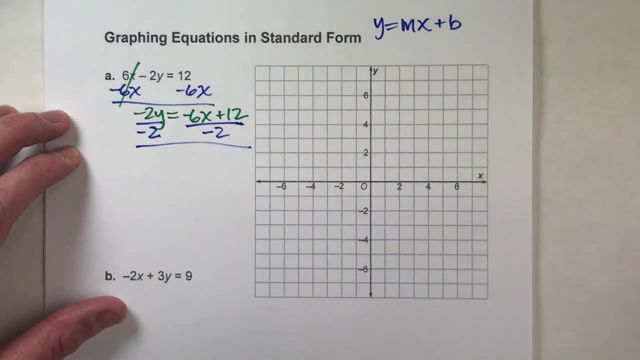 What I do to one side, I have to do to the other and I have to do it to the entire other side, both the negative 6x and the 12. I have to divide the entire thing by negative 2. And when I do that, 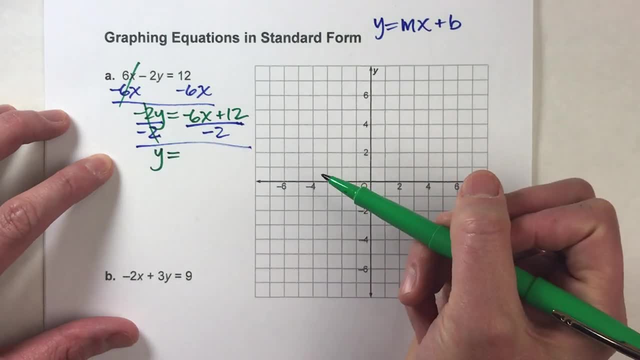 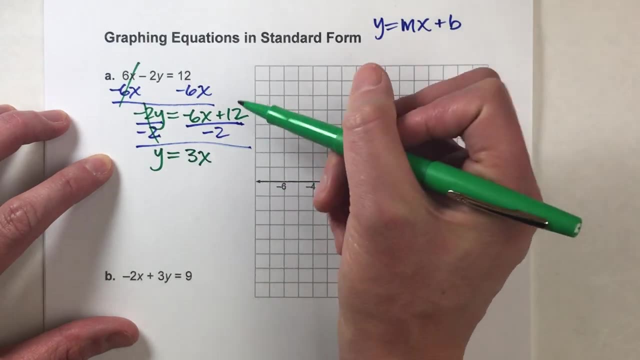 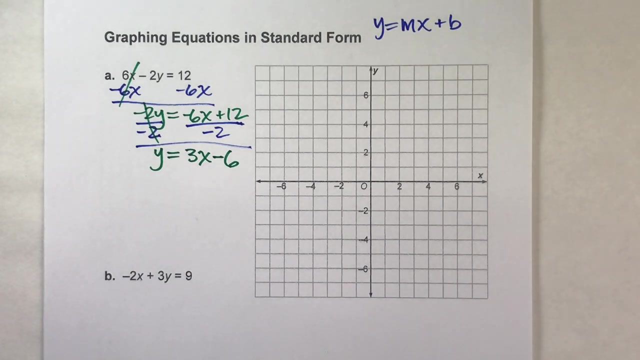 negative 2 is under each other and the y drops down, equals drops down On the other side. negative 6x divided by negative 2 is positive. 3x. positive 12 divided by negative 2 is negative 6.. All right, Now notice, I've got my equation in. 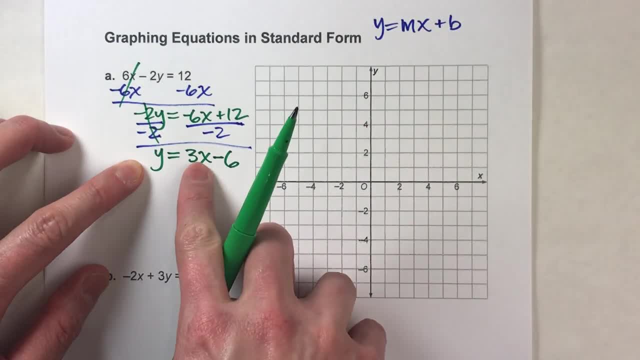 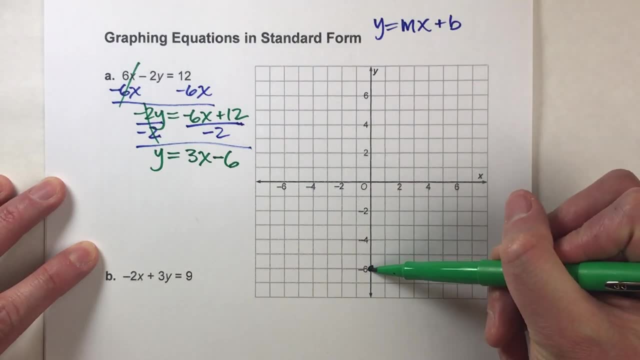 slope-intercept form. now It looks just like this: My slope is 3,, my y-intercept is negative 6.. And now I can graph this: Negative 6 on the y-axis is right here. My slope is 3, or 3 over 1,. 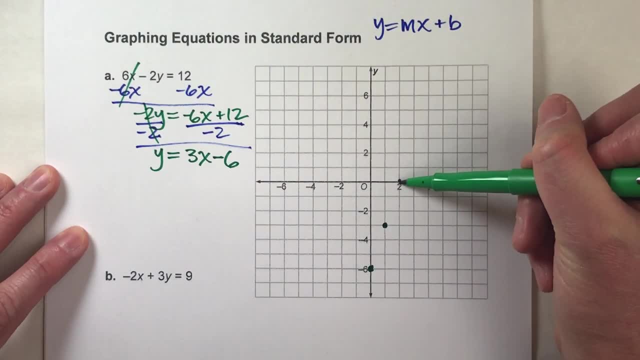 so it's going to go up 3, right 1, plot a point: up 3, right 1, up 3, right 1, up 3, right 1.. There we go, And with my ruler. 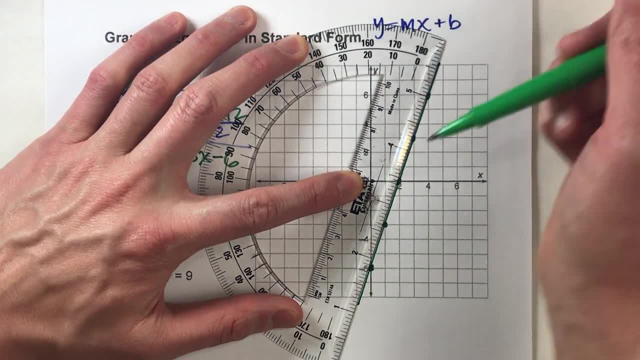 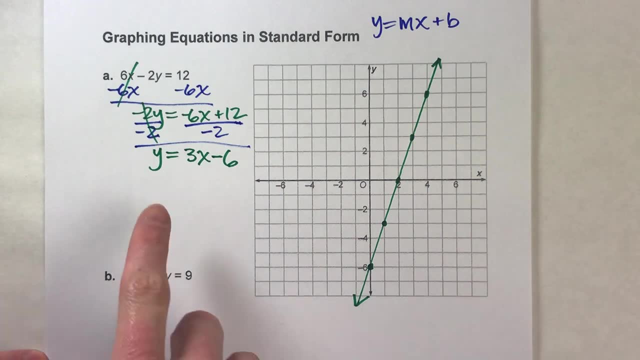 I can draw in my line and there it is All right. So notice, it does take a little bit of work to be able to do that, but once we do those two steps we've got our equation in slope-intercept form. 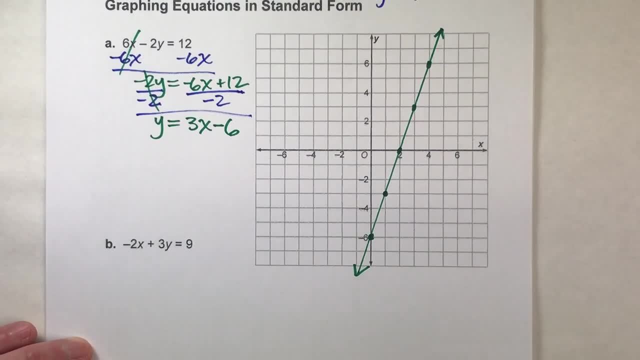 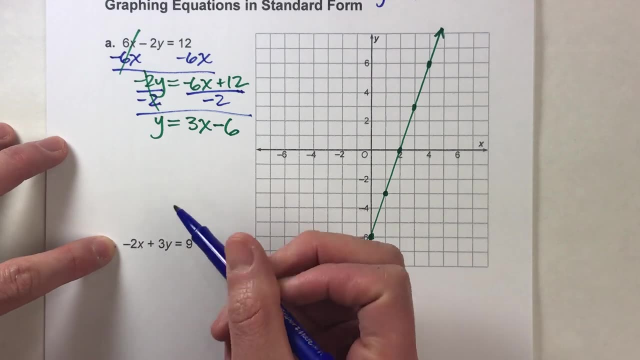 and then we can graph it pretty easily. Let's do the second example now, though. Okay, So we've got negative. 2x plus 3y equals 9.. Again, we want to get y by itself, so I'm going to undo the. 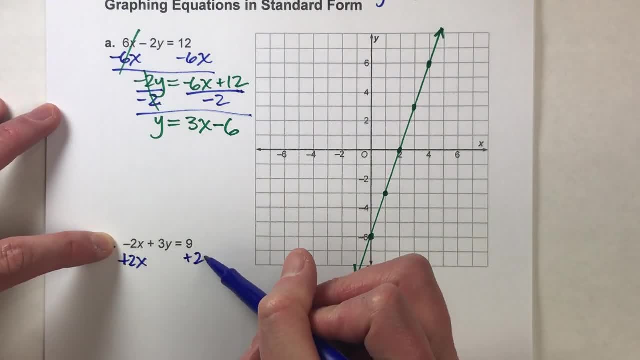 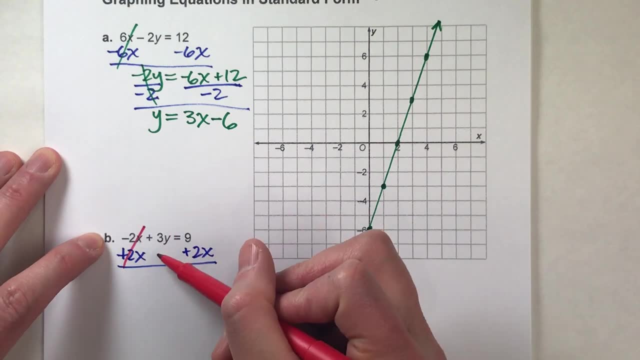 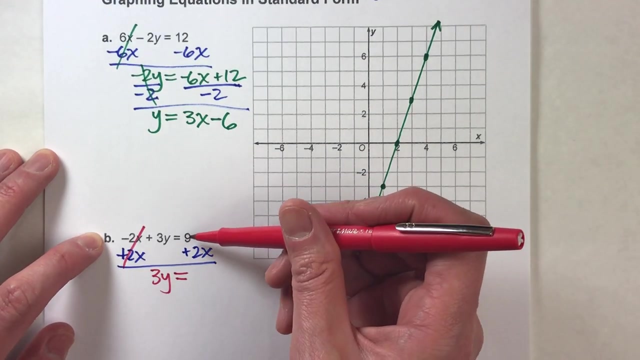 negative 2x by adding 2x to both sides. When I do that, this time I get 2x's undo each other, but the 3y drops down, the equals drops down, and I can't add x's to regular 9s like x's to regular numbers, so I'll keep them separate. 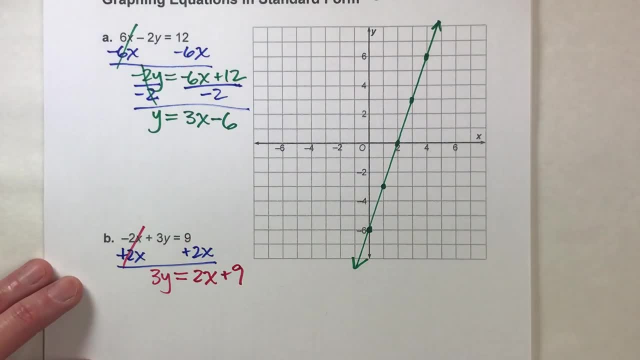 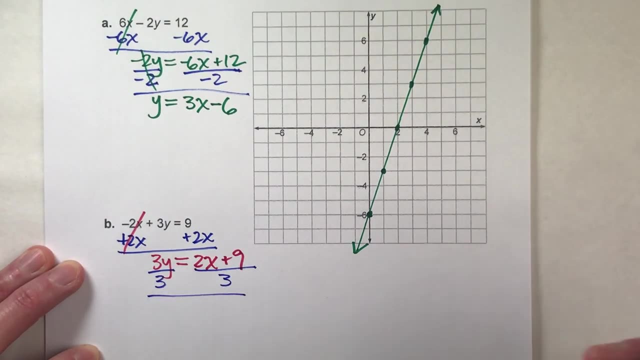 So I've got the 2x here and the positive 9 right there. All right Now to get y, I'll divide both sides by 3, and don't forget, divide the entire other side by 3,, not just part of it, the whole. 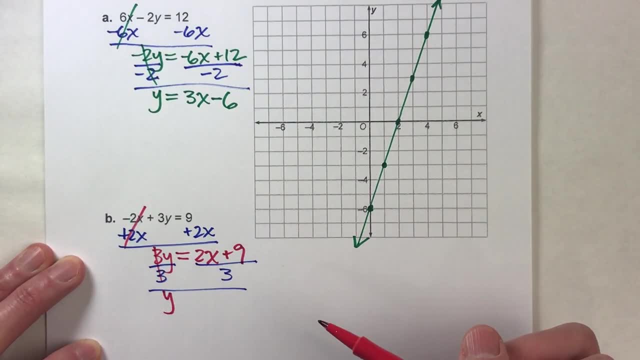 thing: 3's undo each other. y drops down and I get 2x. So I've got negative. 2x plus 3y equals 9, 2x drops down, equals drops down. Now here's where it gets tricky. 2 divided by 3 is not a whole. 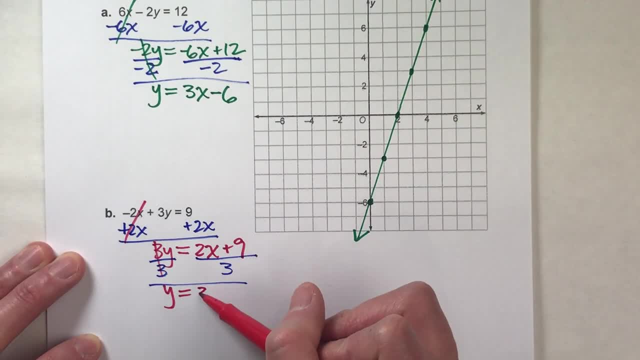 number. so I'm going to keep 2 divided by 3 as 2 thirds, with the x next to it. All right, So keep it as a fraction. It'll be easier to graph. in a second You'll see why. Positive 9 divided by 3. 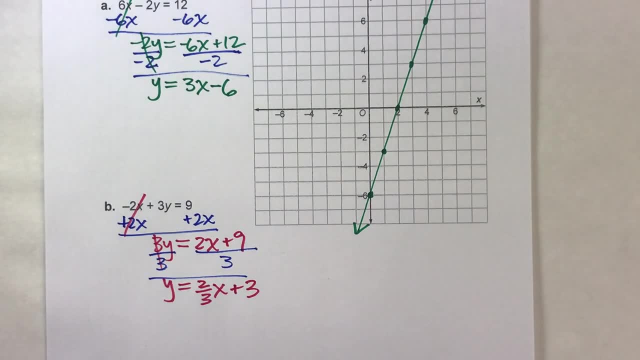 is positive 3.. All right, So notice, I've got it in slope-intercept form now, so now I can easily graph this. My y-intercept is 3, so 3 on the y-axis. I'm going to keep 2 divided by 3 as 2 thirds. 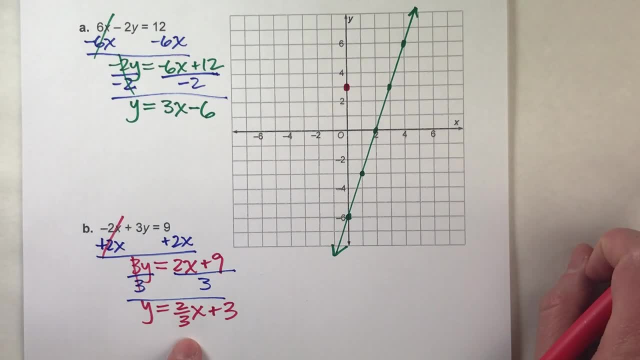 So I'm going to keep 2 divided by 3 as 2 thirds. I'm going to keep 2 divided by 3 as 2 thirds. I'm going to keep 2 divided by 3 as 2 thirds And my slope- because I kept it as a fraction, I can use this as my slope.